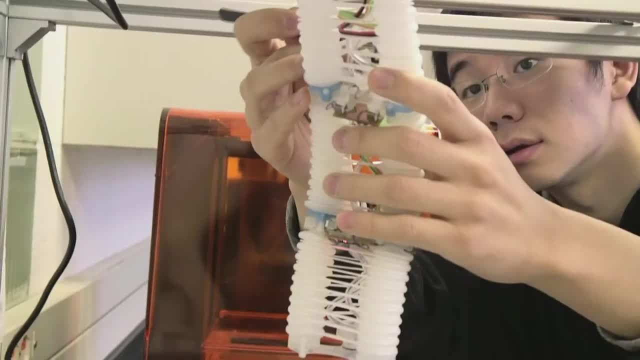 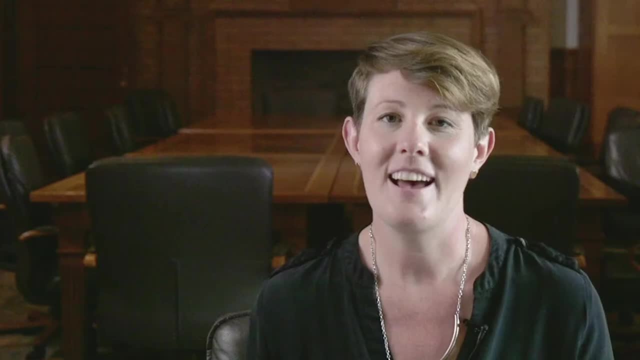 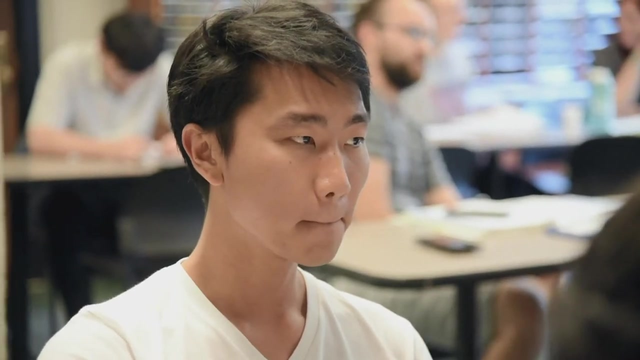 graduating from this major has lots of opportunities across the world. There are international opportunities with verification technology for non-proliferation. We have national laboratories here in the United States and abroad which do research in the context of nuclear energy, nuclear energy systems and nuclear security. There's also industry. 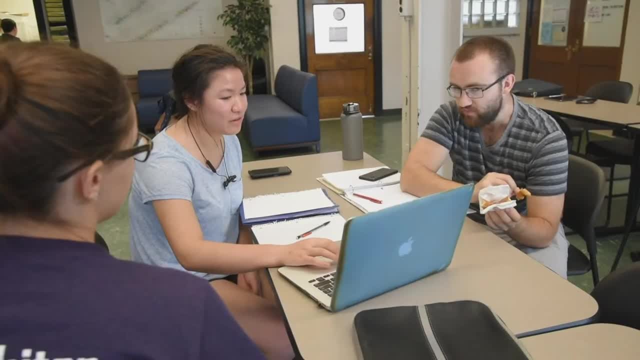 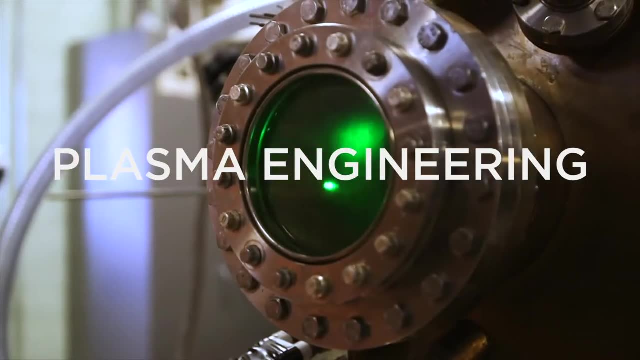 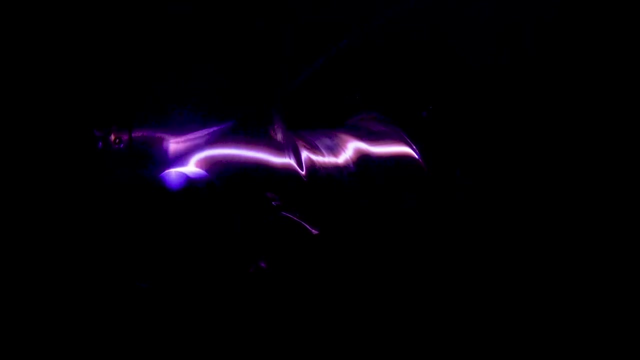 which is really producing this nuclear power, including some very cool new nuclear startups that have great ideas for the next generation of nuclear reactors. Plasmas are the fourth state of nature: Solids, liquids, gases And then plasmas- hot ionized gases. 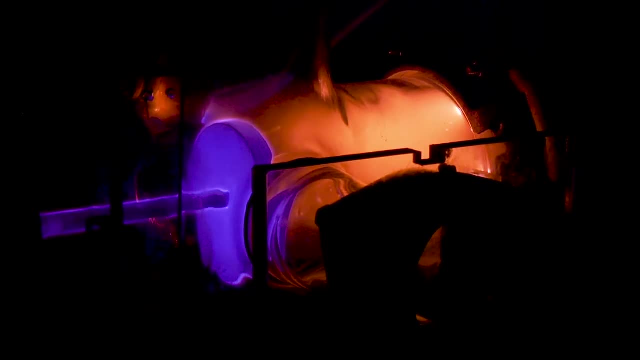 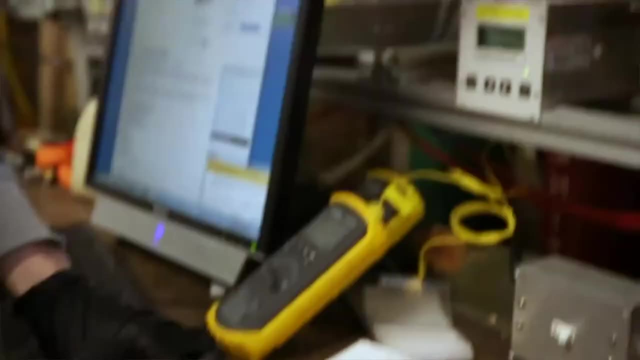 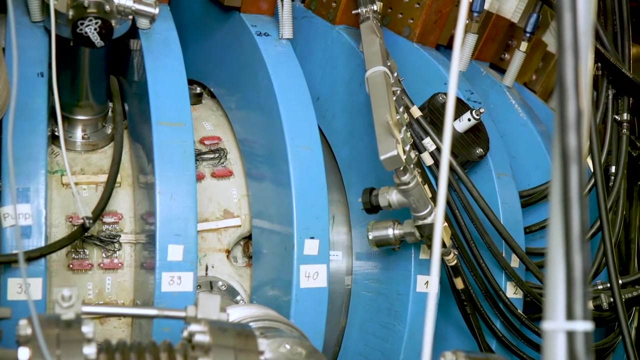 And the thing is, you can use plasmas to make things, And that's what the field of plasma engineering is all about: How you can utilize plasmas to produce goods, products and even energy- fusion energy, Like what this machine makes behind me, Hydra. 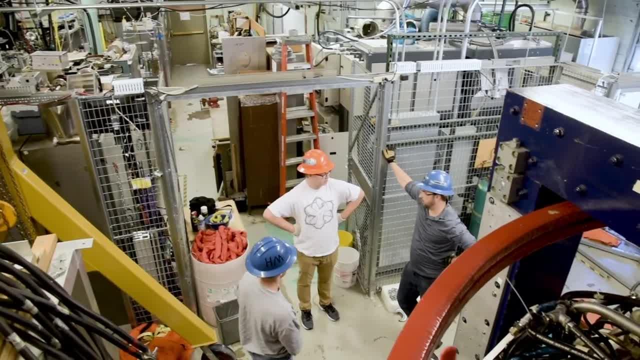 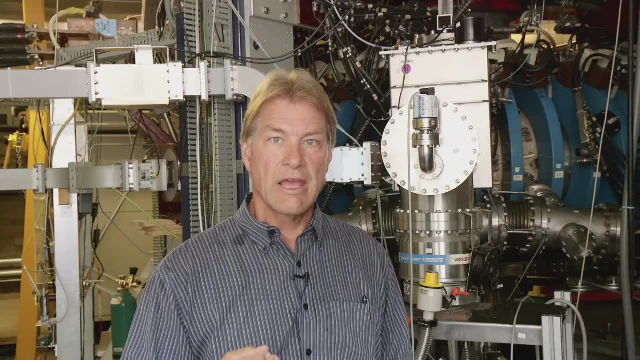 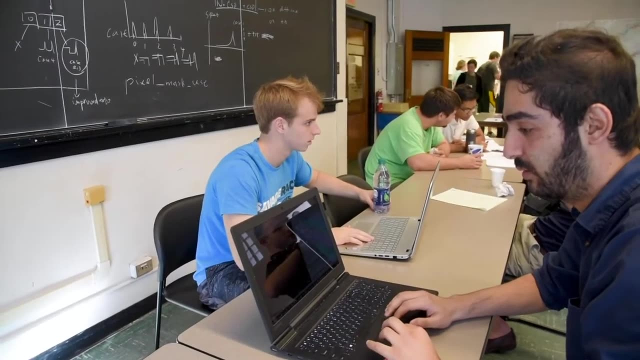 Fusion is just scratching the surface, Being able to use a plasma to manufacture things, to process, to make stuff. In fact, everything in microelectronics, everything that makes cell phones, computers, game consoles possible, every computer chip was made using a plasma. 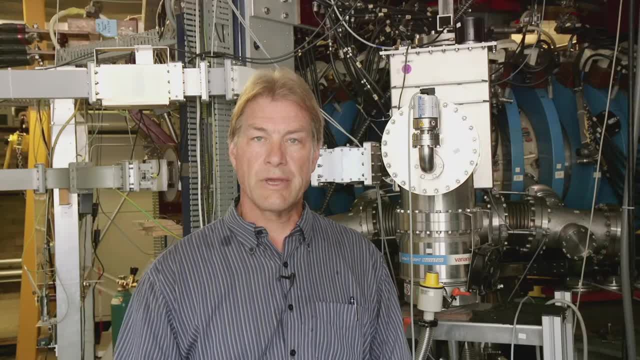 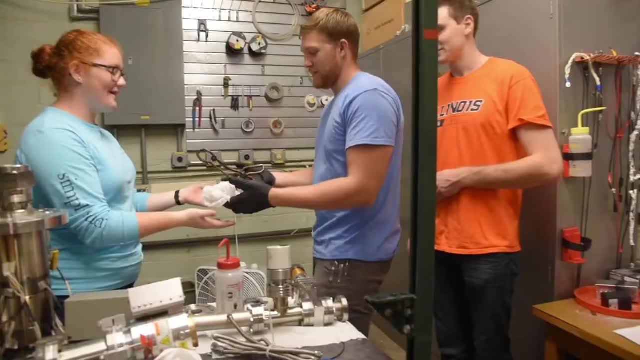 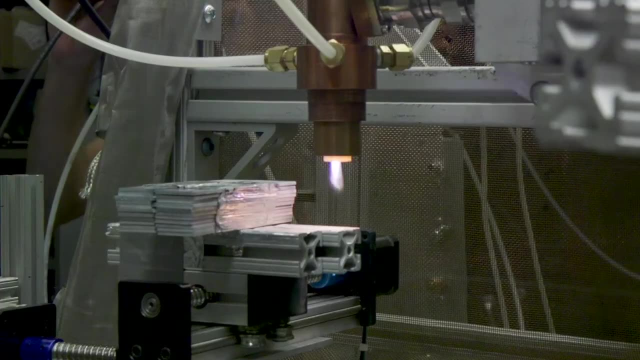 Companies from the whole range of the semiconductor manufacturing industry want to hire as many of our graduates as they can at all the levels: Bachelors, Masters or PhD, Automotive, aerospace or even agriculture. Plasma engineers are needed throughout the entire workforce. 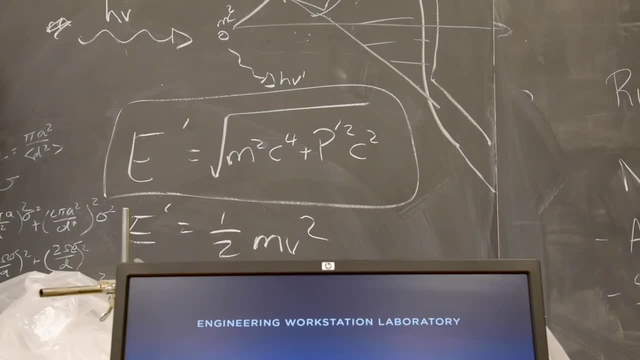 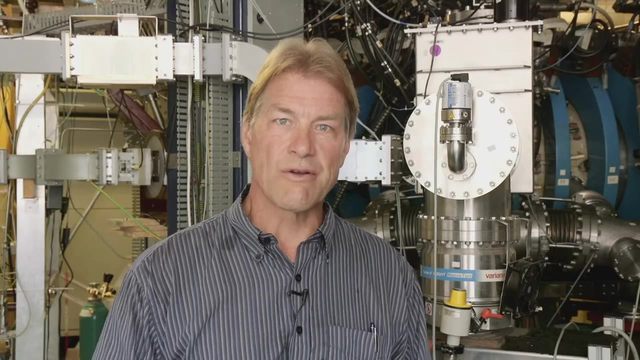 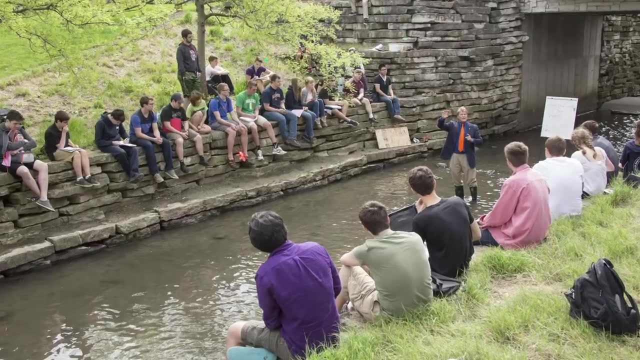 So what skills do you need to succeed in our program? Math and science, And a desire to know and think about how things work. Plasmas are the field for you, Whether you want to save the world by making fusion energy a possible clean source for the future. 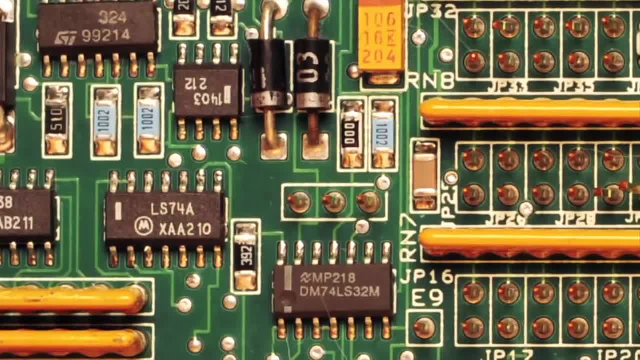 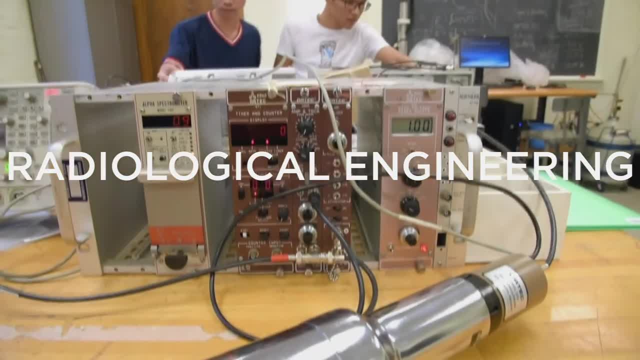 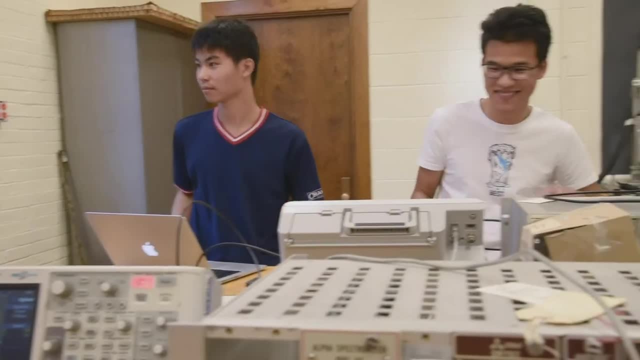 Or whether you just want to make the world a better place by making electronics and computer chips even faster, even better and even cheaper. Students in radiological science share with students in nuclear and plasma engineering the same passion for science and research. They need to have a strong background in math and physics.